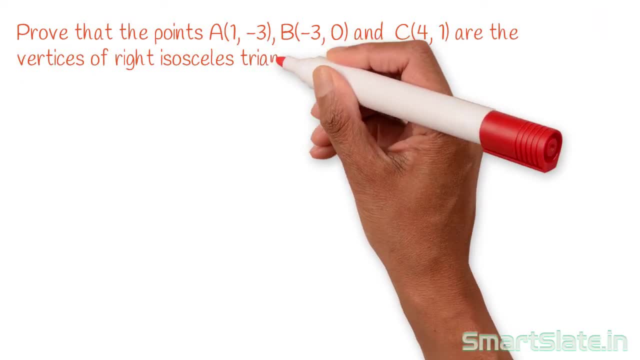 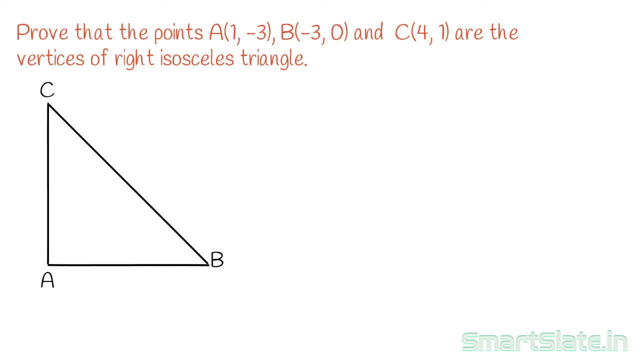 and 1 are vertices of right isosceles triangle. The Iso Cela's triangle has two equal sides. If we prove distance between any of two sets of points is equal, then we can say: this points forms an Iso Cela's triangle and if square of longest side is equal to addition of squares, 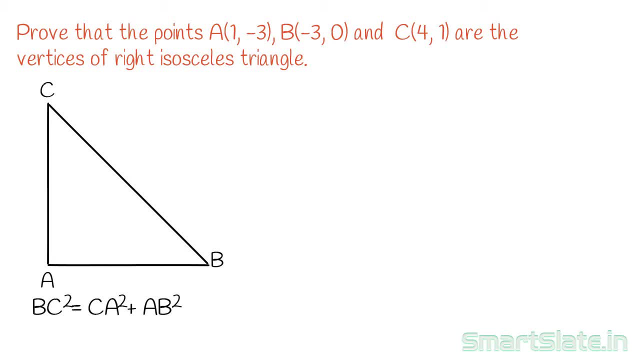 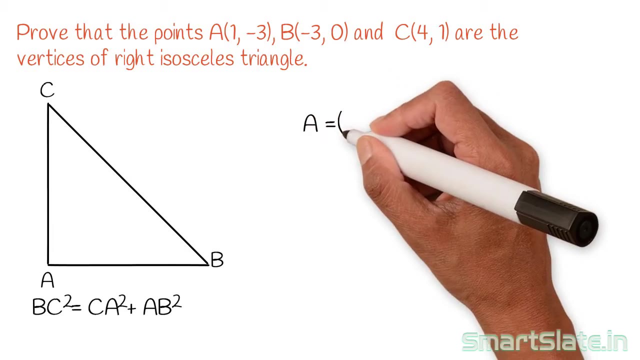 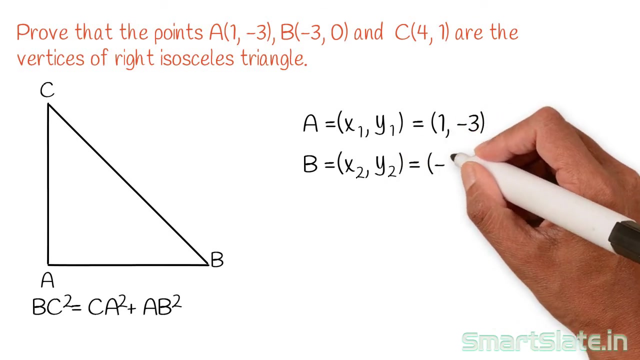 of other two sides, then triangle is right angled triangle according to Pythagoras theorem. Calculus: calculate distance AB, BC and CA using distance formula. Consider point A: x1, y1, which is equal to 1 minus 3.. Point B is x2, y2, which is equal to minus 3 and 0.. And point C is: 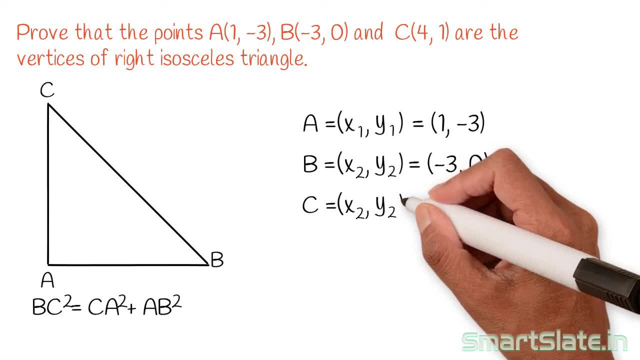 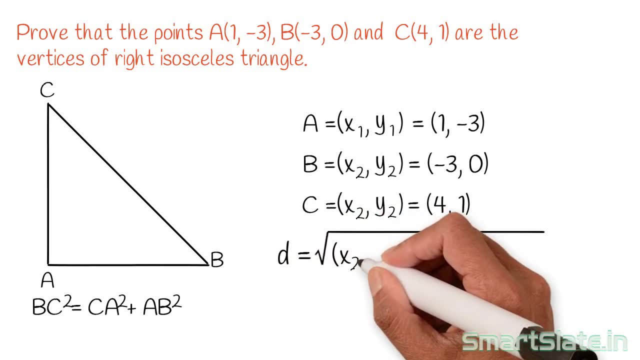 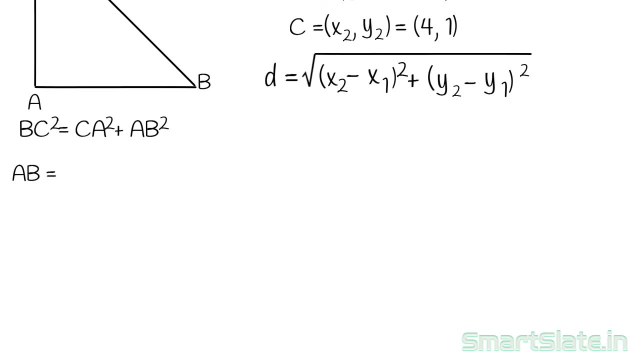 also x2, y2 and the values are 4 and 1.. We are supposed to calculate the distance using the formula square root of x2 minus x1 square plus y2 minus y1 square. First, calculate AB. Replace x1, y1 and x2, y2 with values. It is square root of minus 3 minus 1 square plus. 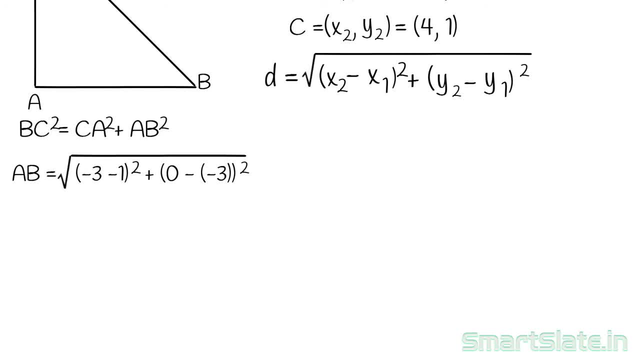 0 minus minus 3 square, It is square root of minus 4 square plus 3 square, which is nothing but square root of 16 plus 9, which is square root of 25.. So the distance of AB is 5 units. Now let's calculate BC: Square root of 4 minus minus. 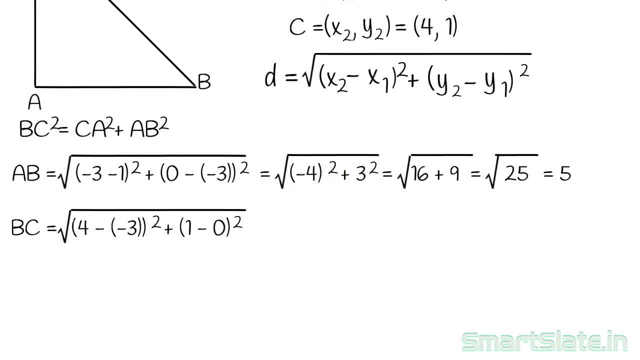 3 square plus 1 minus 0 square, It is square root of 7 square plus 1 square. 7 square plus 1 square is 49 plus 1.. It is square root of 50.. Now calculate CA. It is square root of. 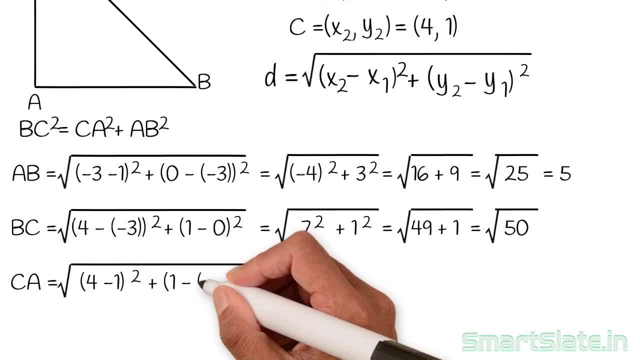 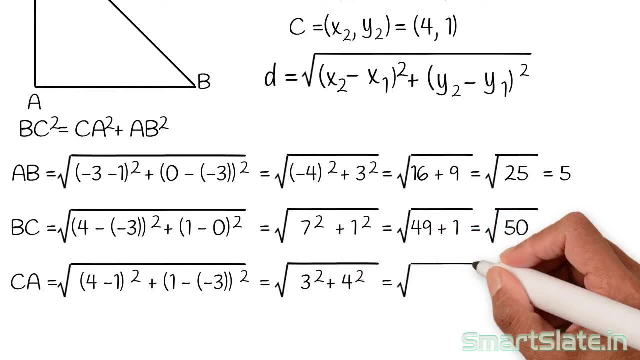 4 minus 1 square plus 1 minus minus 3 square, It is square root of 3 square plus 4 square. 3 square plus 4 square is 9 plus 16. It is square root of 25.. So the distance between C and A is 5 units Since AB. 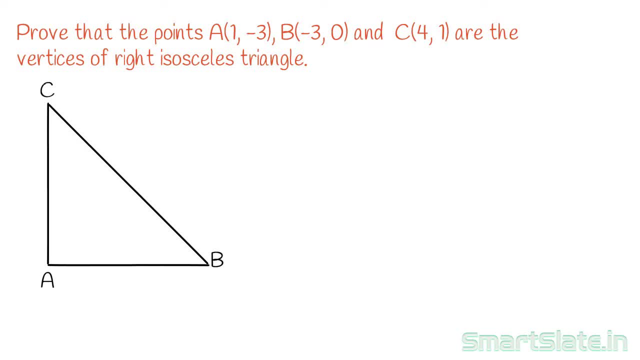 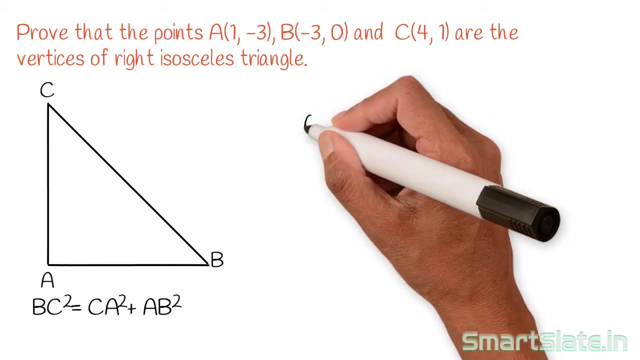 we can say: these points forms an isosceles triangle, and if square of longest side is equal to addition of squares of other two sides, then triangle is a right angled triangle according to Pythagoras theorem. Calculus distance AB, BC and CA using distance formula. consider point a, x1, y1, which is: 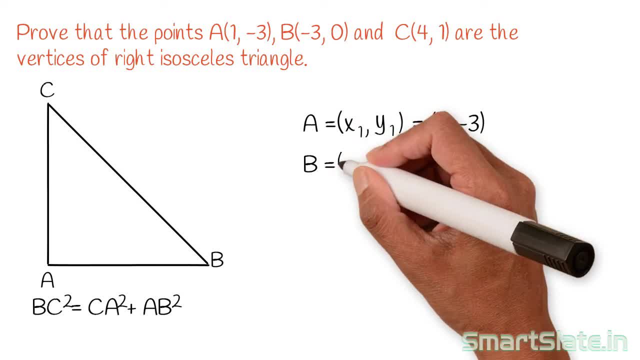 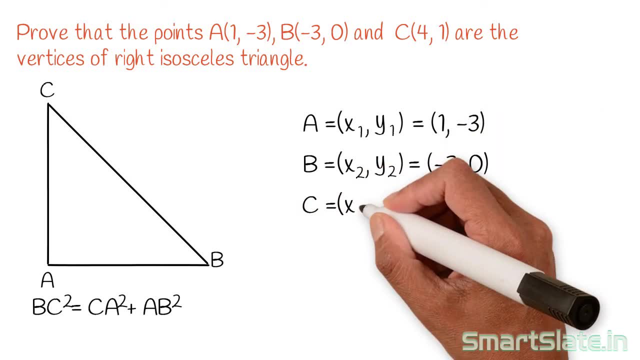 equal to 1 minus 3, point B is x2- y2, which is equal to minus 3 and 0, and point C is also x2- y2 and the values are 4 and 1. we are supposed to calculate the distance using the formula square root of x2 minus x1 squared. 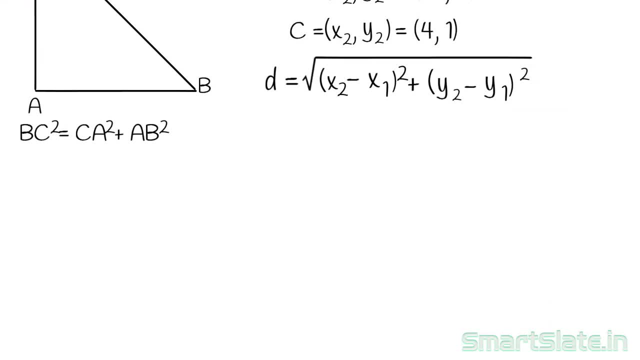 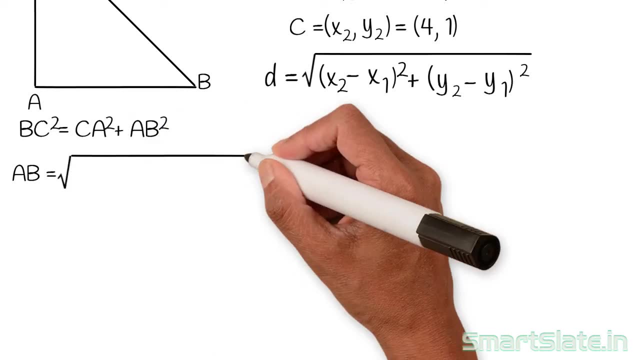 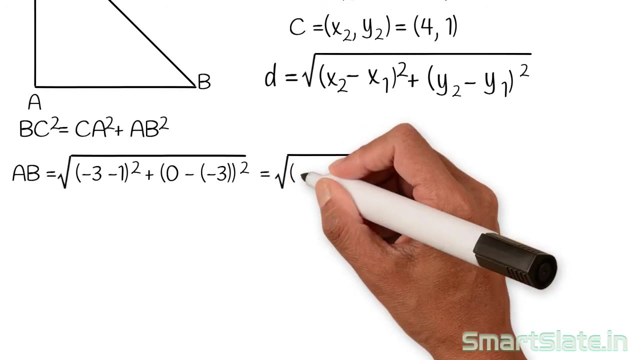 plus y2 minus y1 Square. first calculate AB. replace x1- y1 and x2- y2 with values. it is square root of minus 3 minus 1 square plus 0 minus minus 3 square. it is square root of minus 4 square plus 3 square, which is nothing. 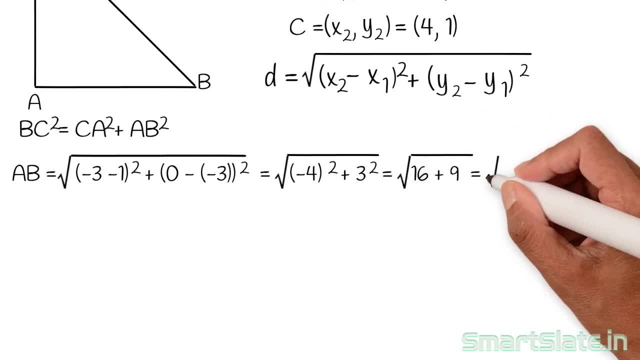 but square root of 16 plus 9, which is square root of 25. so the distance of AB is 5 units only. so the distance of now, let's calculate BC: square root of 4 minus minus 3, square plus 1 minus 0. 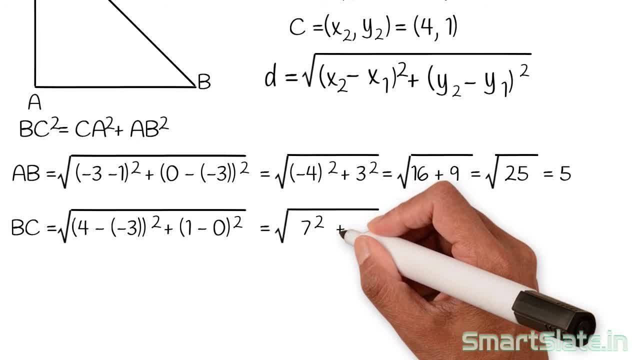 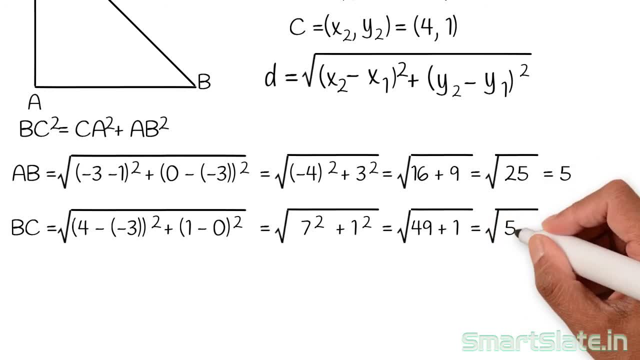 square. it is square root of 7 square plus 1 square. 7 square plus 1 square is 49 plus 1. it is square root of 50. now calculate CA. it is square root of 4 minus 1 square plus 1 minus minus 3 square. it is square root of 3 square. 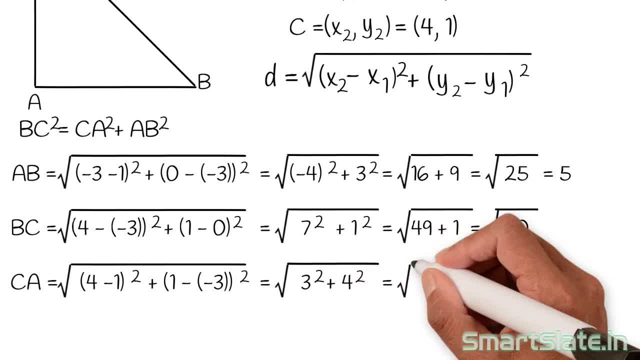 plus 4 square, 3 square plus 4 square is 9 plus 16. it is square root of 25. so the distance between C and A is 5 units. since AB and CA are equal, the triangle which consists these points is a isosceles triangle. now let's try to. 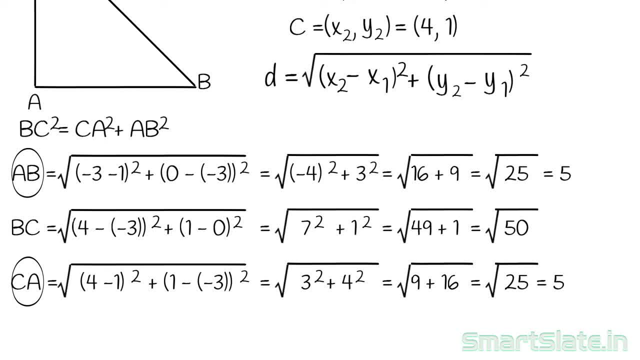 prove that it is a right angle to triangle. now let's try to prove that it is a right angle to triangle. now let's try to. according to Pythagoras theorem, if square of a longest side is equal to addition of squares of other two sides, then triangle has to be right angle.